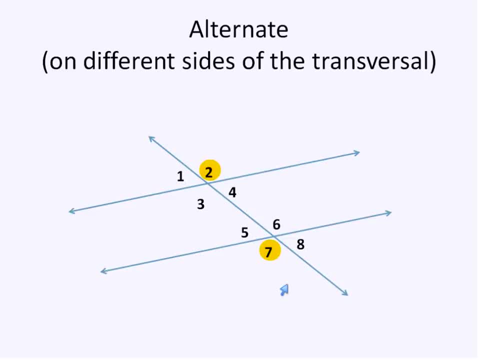 the two parallel lines, So our transversal. anything on opposite sides of the transversal are called alternate angles, So you could also have this like: 2 and 5 are alternate angles because they're on opposite sides of the transversal. 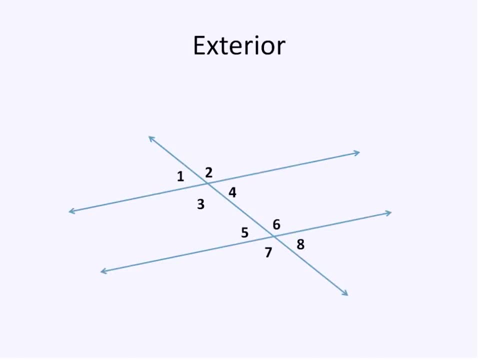 We'll also talk about exterior and interior angles. Exterior angles are angles that are on the outside of the parallel lines. I've represented that with these light blue shaded sections. Anything on the outside of the parallel lines are going to be called exterior angles. 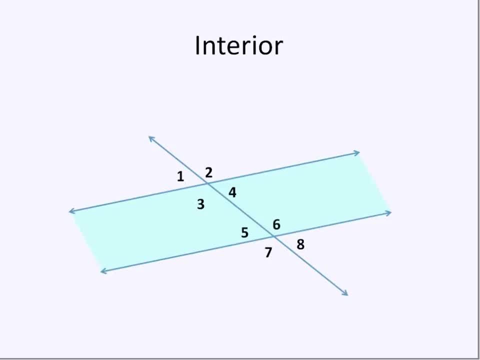 Anything on the inside of the parallel lines will be called interior angles. It seems pretty straightforward, but I just want to be clear of where the exterior, interior, and then also the alternate that we talked about. So the next part, then, of course, is to put these two ideas together. 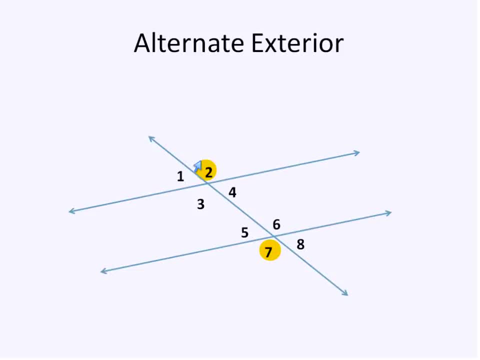 An alternate exterior angle are the two angles that are on different sides of the transversal, like 2 and 7, and they're on the outside of the parallel lines, the exterior of the parallel lines. Those are alternate exterior angles. The other example of alternate exterior angles: 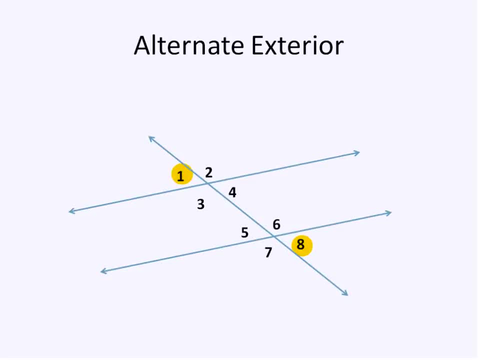 is angle 1 and angle 8.. They are on the different sides of the transversal exterior or the outside of the parallel lines. The neat thing, property of alternate exterior angles, is that they're congruent, They're the same measurement and they look the same. Look the measurement of angle 1, here it's. 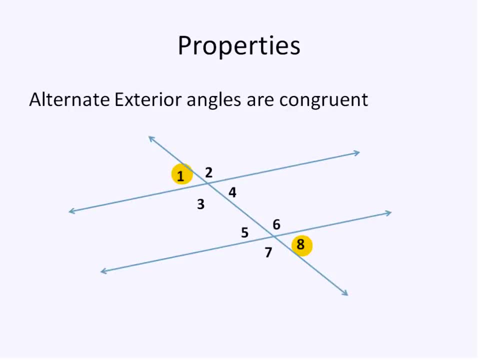 definitely an acute angle and you see measurement of angle 8, it looks the same and they are the same Alternate exterior angles are congruent. So that's one property and one way that, essentially, if you know one of these eight angles, you 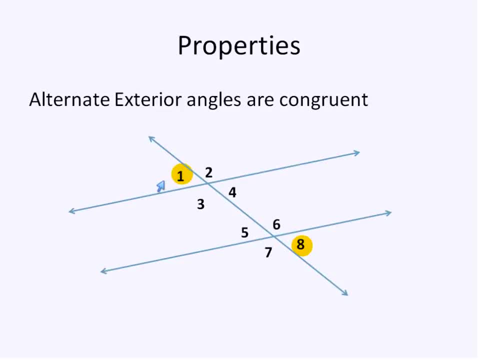 can tell what all of the other eight ones' angles and measurements are, And that's neat and one of the ways you know that is because alternate exterior angles are congruent. Alright, Now that we've talked about alternate exterior, where do you think the alternate? 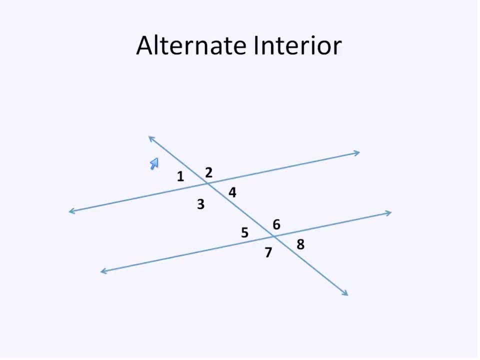 interior angles might be. We see the word alternate, which means they have to be on different sides of this transversal. One will be on this side and one will be on this side, And we see the word interior, which means they'll be on different sides of this transversal. 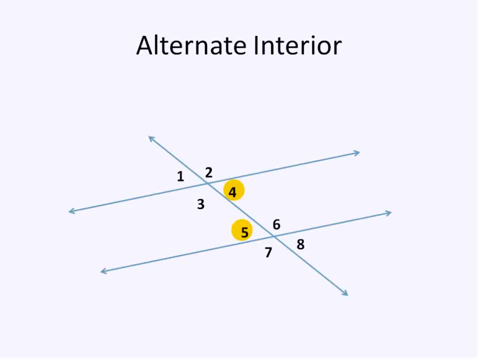 You can tell, be on the inside of the parallel lines. So one example of alternate interior angles is 4 and 5, angle 4 and angle 5.. The other example is angle 3 and angle 6. And just like alternate, 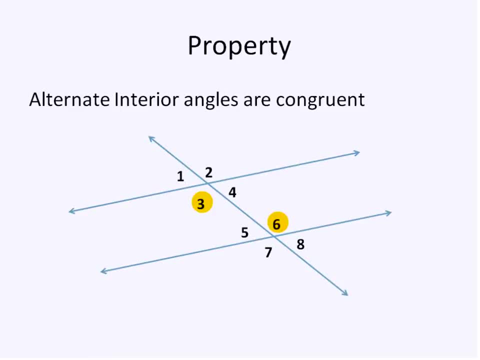 exterior angles, we know that alternate interior angles are also congruent. So angle 3 is equal to angle 6.. Angle 4 is equal to angle 5 because they are alternate interior angles, Corresponding angles for me, what I like to do when I'm thinking about corresponding 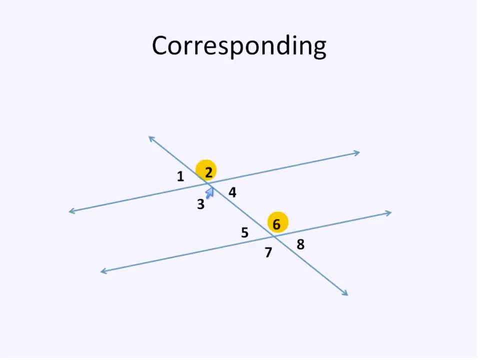 angles is I like to look at just one set of four angles at a time. So I look at this set of angles and you can put a circle around it or a square around it or something, just to say I'm looking at just this section, separate from the other ones, And then put 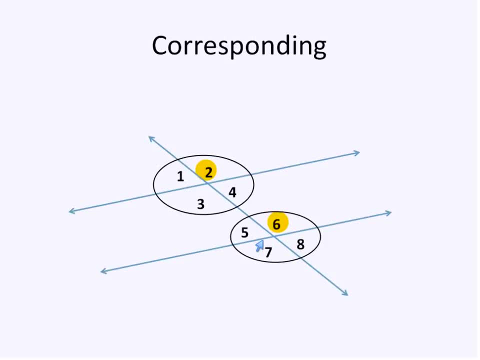 a similar circle around that and basically what corresponds to the other angles is the same. So what corresponding angles means is, if you're only looking at this circle and this circle, they're in the same exact place. So corresponding angles are angles 2 and 6.. Can you see another set of corresponding angles? 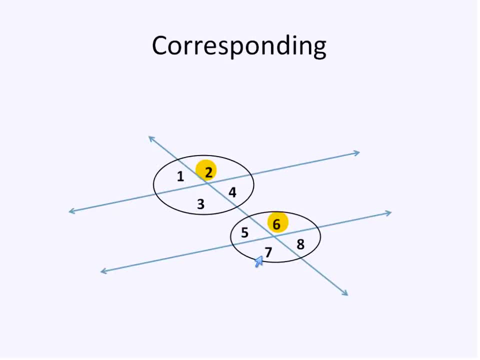 Perhaps you notice that 1 and 5 are corresponding angles, 3 and 7 are corresponding angles And angle 4 and 8 are the last set of corresponding angles. So I'm going to represent them by color coding them here To show that these are the corresponding angles, And for me it's easiest to just put. 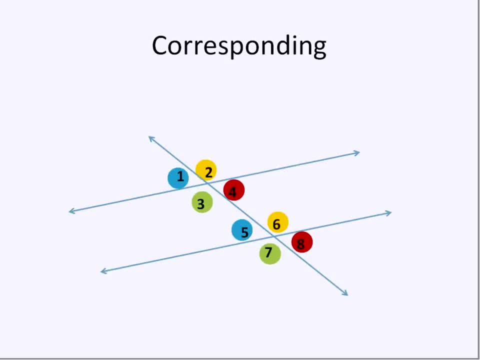 a circle around that. You can also color code it, if that helps, and identify which angles are corresponding. Now one property about corresponding angles- you may have already guessed- is that the corresponding angles are congruent. All right, Angle 2 is the. 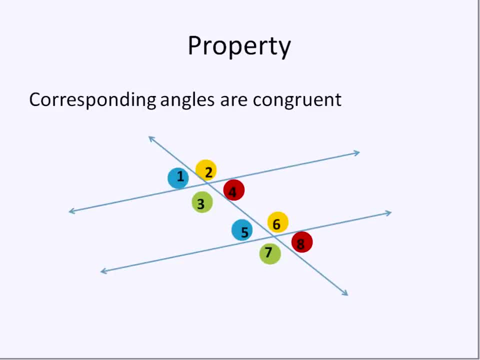 same measurement as angle 6.. Angle 1 is the same measurement as angle 5. So corresponding are congruent, they have the same measurement, Alright. The next set of angles are called adjacent angles, And adjacent just means next to, so basically any two angles that are next to. 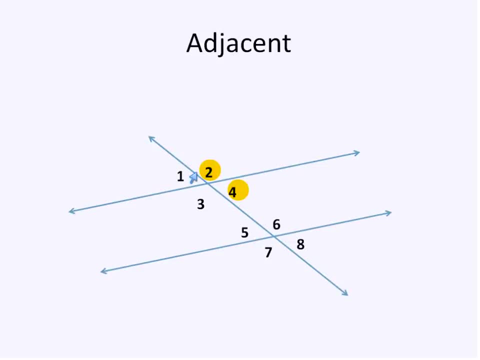 each other. 2 is next to angle 4.. 2 is also next to angle 1.. We could have highlighted 2 and 1, they're adjacent angles. 2 and 4 are adjacent angles. Here's another example: 5 and 6,.